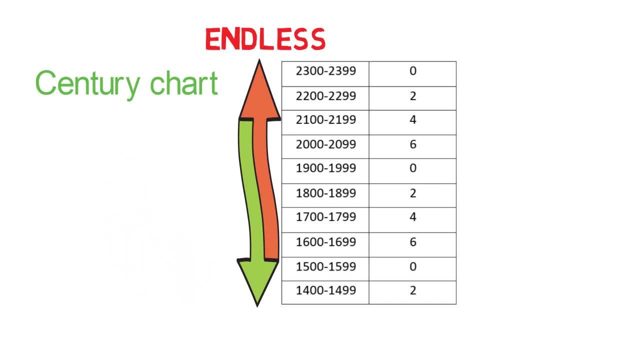 But how to use this chart. In the date we have year, First see the year belongs to which century. Then the code of that century will be the code of that year. By the way, everything will be clear when we will go through the examples. 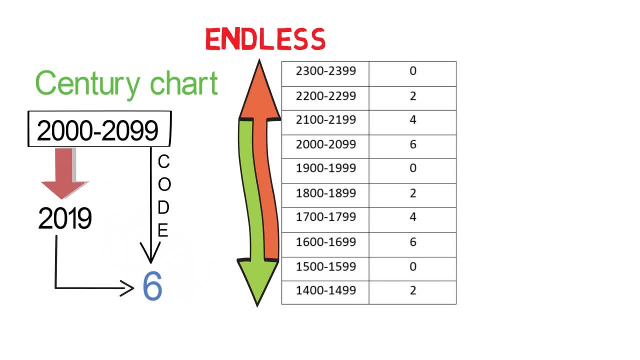 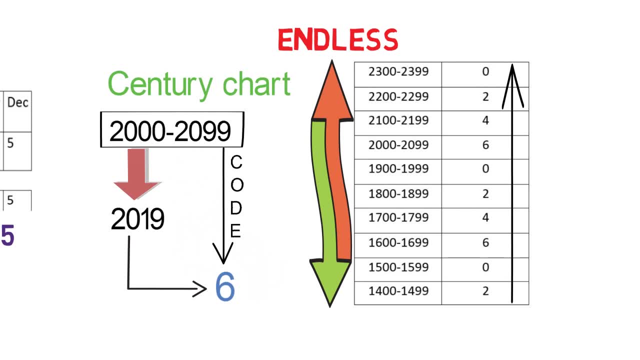 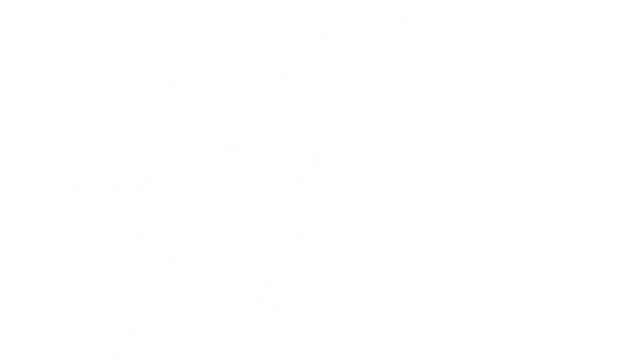 Now how to remember the century codes. You may have already noticed that there is a repetitive pattern in the codes, which are arranged vertically From the below. these are repeatedly like 2064, again 2064, and so on. So these are the 3 charts that you will require to solve the problem. 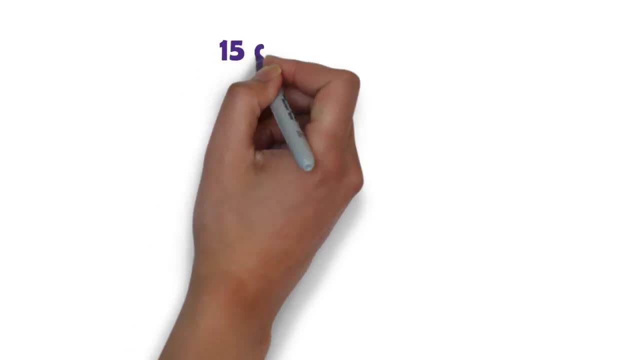 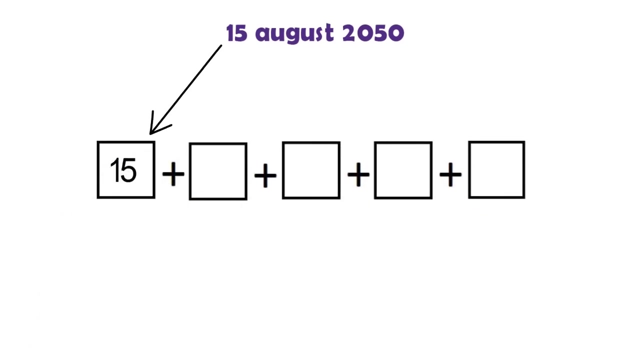 Ok, let's start. Take any random date To solve it. we need to do only one addition and one division. Let's do the addition first. We have to add 5 numbers: First, the date itself. Second, the month code. 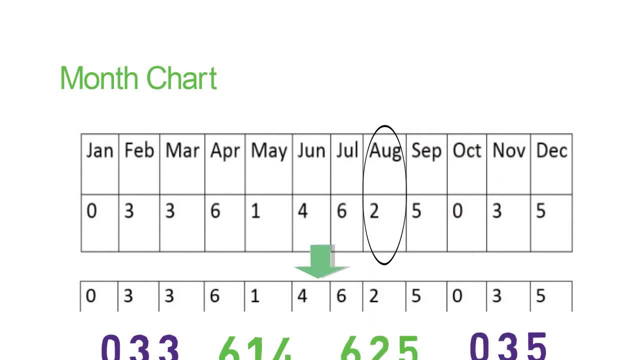 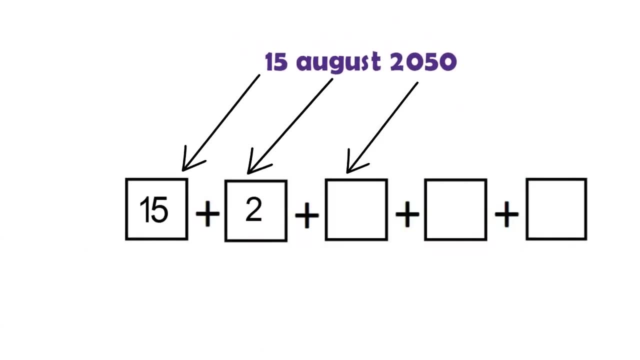 From the month chart for this problem, write code for August, which is 2.. Third, the century code For 2050, the century is 21st And from the century chart we get the code 6 for 21st century. 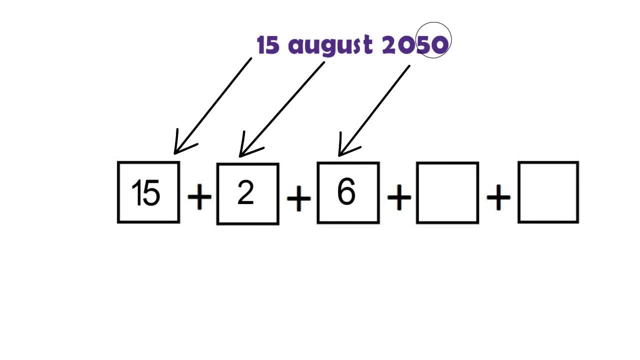 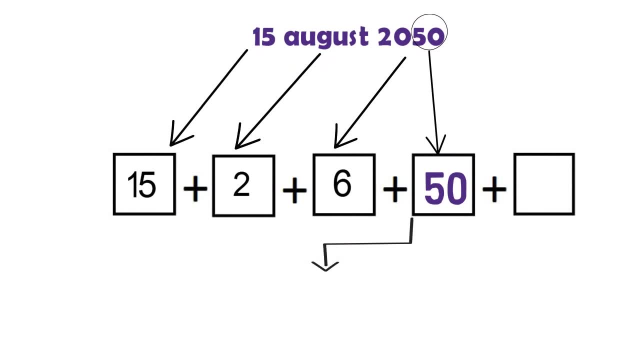 The fourth number is the last 2 digit of the year, that is, 50.. And the fifth number that we have to add is the quotient of 50. If we divide this 50 by 4.. Remember, only the quotient is to be taken. 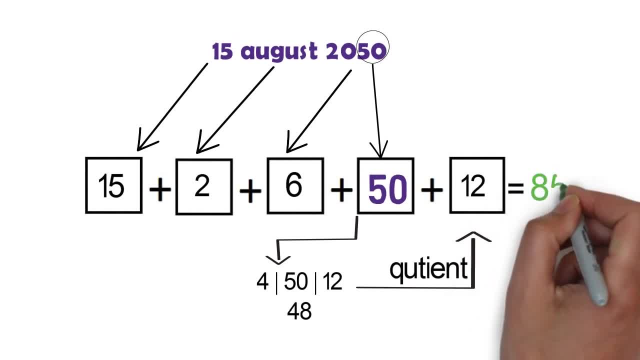 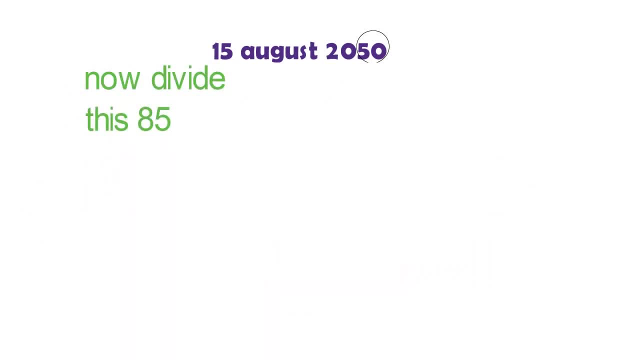 Now add these 5 numbers and we get 85. The second step of this problem is the division. Divide this 85 by 7. This time, take the remainder only And guess what We are done with the problem, As this remainder 1 is the final. 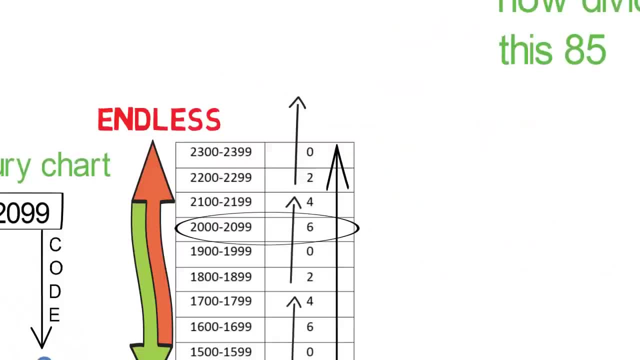 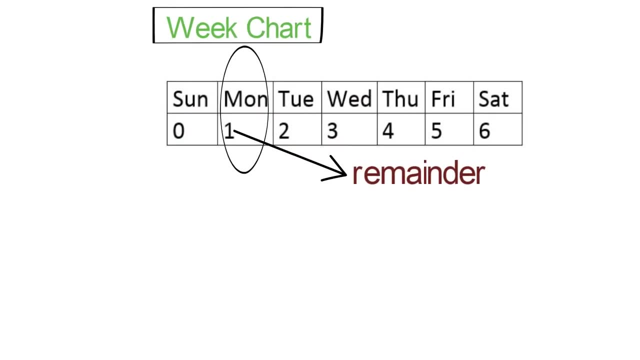 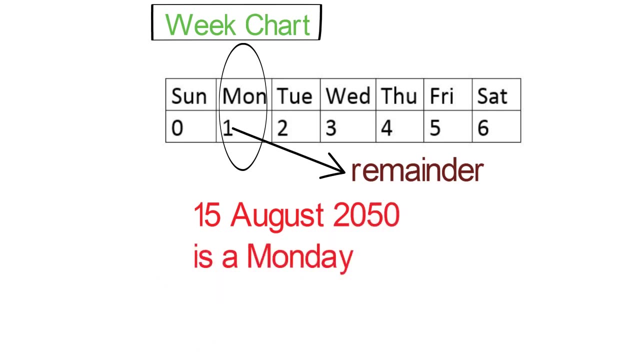 Clue To find the weekday: see the week chart Here. this remainder 1 refers to Monday. So our date, 15th August 2050, is a Monday. This way we have completed the general method of this problem.